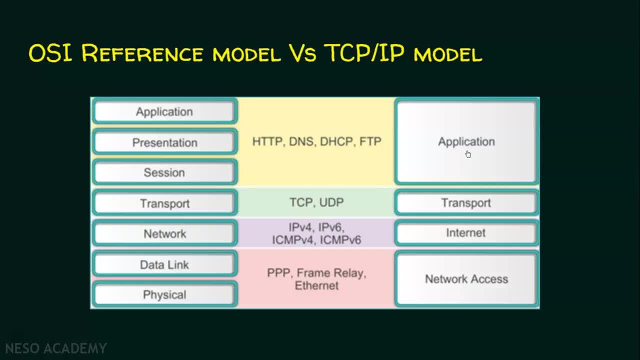 Actually, TCP IP model was developed prior to the OSI model, So this is the actual implemented model. and this is just a reference model, just a guideline. in some books TCP IP model is shown with five layers, So no problem whether it is a five-layered architecture. 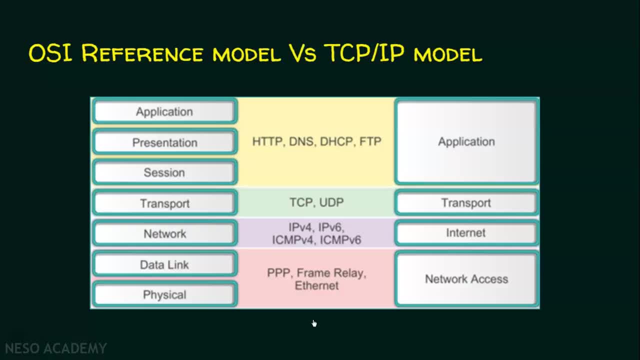 or four layered architecture, the functionality still remains the same. If you want TCP IP model with four layers, You can use any of these sockets. If you want TCP IP model with four layers, You can use any of these sockets with five layers. just break this network access layer. 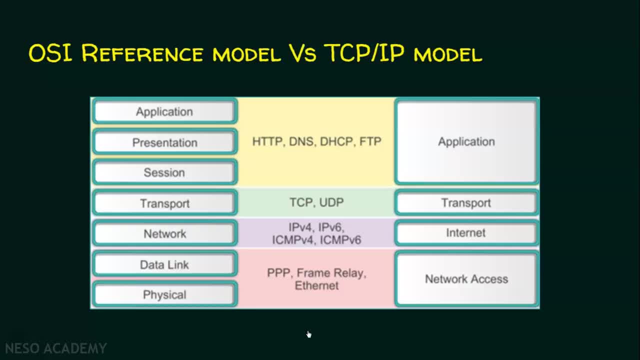 into physical layer separately and data link layer separately. There are some protocols that are there in every layer of the TCP IP model Because that protocol only does the functionality of that layer. If you take network access layer, point to point protocol simply PPP. 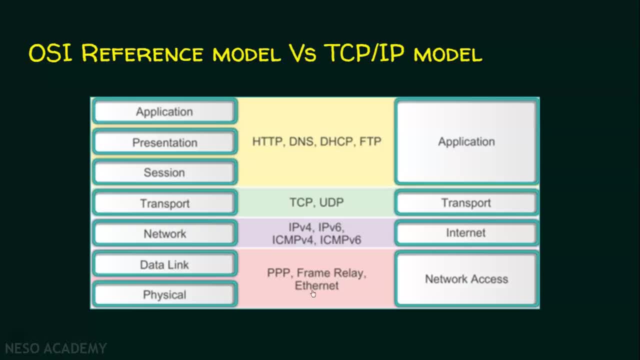 Frame relay is very popular in network access layer. Ethernet is a very popular protocol in the network access layer. In coming to the internet layer, we have IP protocol. IP means it's simply IPv4 or IPv6, ICMPv4 and ICMPv6. 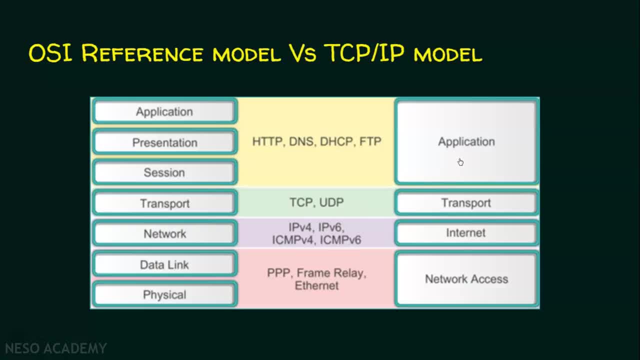 In the transport layer we have TCP and UDP. In the application layer we have HTTP, DNS, DHCP and FTP. It's quite difficult to understand all the protocols now, even the expansions, but let it be as such. Anyway, we are going to talk about these protocols. 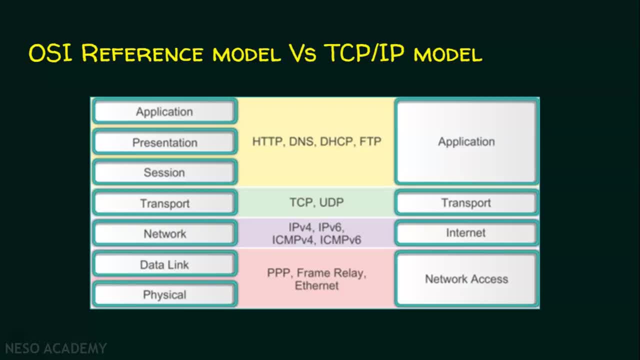 elaborately. in the end We are going to cover the entire course, so no worries. For time being we will just have the expansion of this protocol and the basic working of these protocols. Now we will see the actual TCP IP model. So the TCP IP model has four layers. 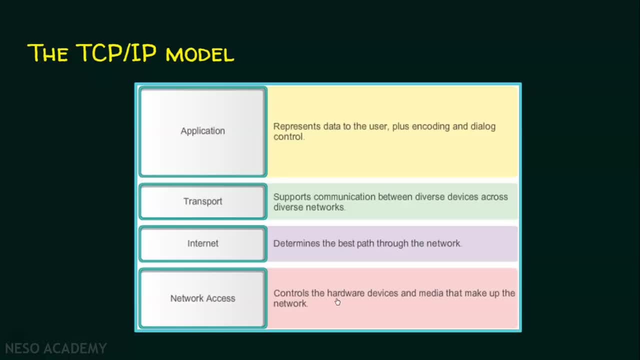 Network access layer, so it controls the hardware, because physical layer is a part of network access layer, So it controls the hardware devices and media that make up the network. And coming to the internet layer, this is the network layer actually, So it determines the best path through the network. 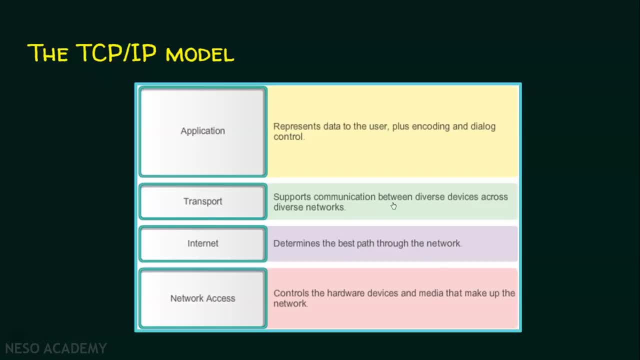 And coming to the transport layer, it supports communication between diverse devices across diverse network. Simply, transport layer deals with process to process communication. And coming to the application layer, this layer is actually dealing with the users, So representing the data to the user, plus encoding and dialog control. 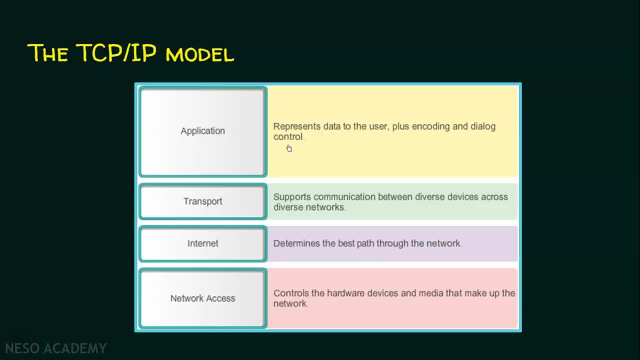 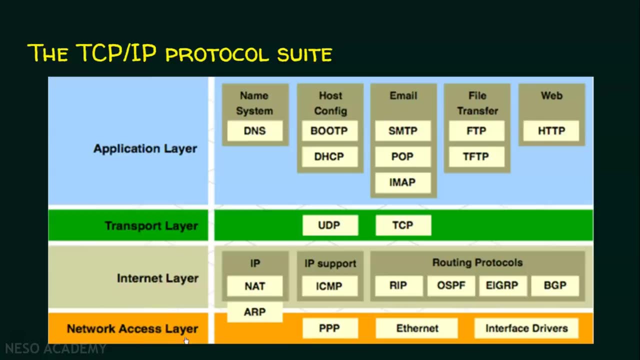 simply the functionalities of application layer, presentation layer and session layer are combined into a single layer. Now we will see the TCP IP protocol suite. So the network access layer has protocols like point to point protocol, PPP, Ethernet protocol. it is a very popular protocol for LAN technologies. 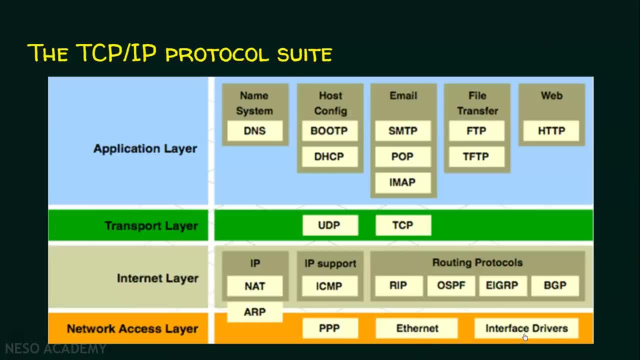 to be precise, wired LAN technologies and there are many interface drivers that work on this network access layer. And coming to the internet layer, the routing protocols will come in the internet layer. We know very well router is a device that works with the network layer. 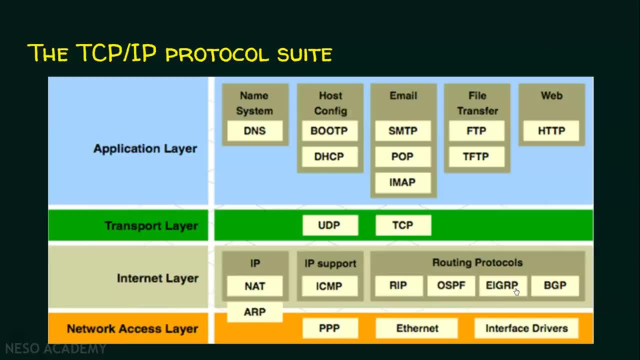 Routing protocols like RIP, OSPF, EIGAR, IRP, BGP- we will talk about these protocols elaborately in the network layer part- and we have IP support protocol like ICMP and NAT, Network Address Translation. And coming to the transport layer, the widely used transport layer protocols are: 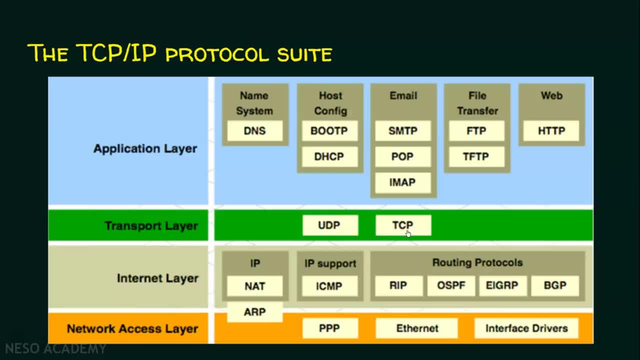 TCP and UDP. TCP means transmission control protocol and UDP means user data grant protocol, So any application will use either TCP or UDP. We will talk about these protocols- transport layer protocols- in the upcoming lectures, in the network layer part And coming to the application layer. 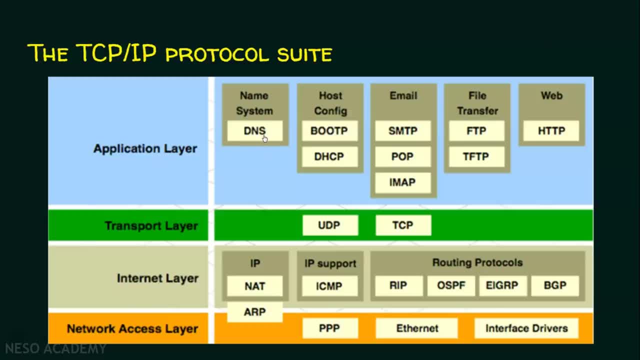 protocol. we have domain name servers or domain name system, that is the name system. There are host configuration protocols like bootp or bootstrap protocol, dynamic host configuration protocol or simply DHCP, and we have email related protocols like simple mail transfer protocol, SMTP. 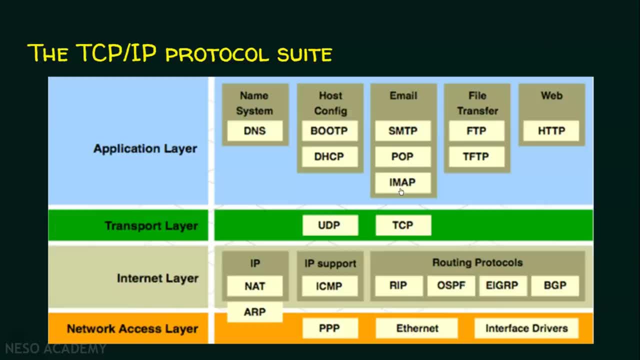 post office protocol or simply POP, or internet message access protocol or simply IMAP, And we have file transfer protocols like FTP file transfer protocol and trivial file transfer protocol, And to access the web or web pages we have HTTP. So these are the popular protocols in the 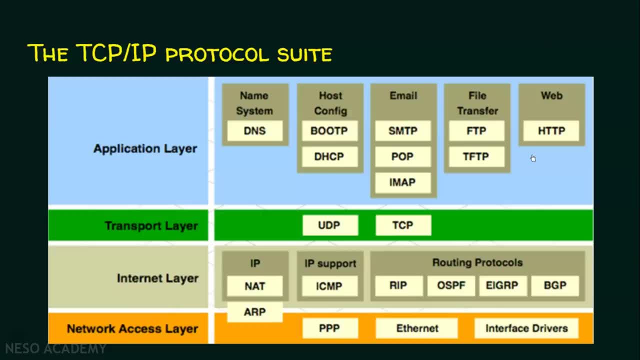 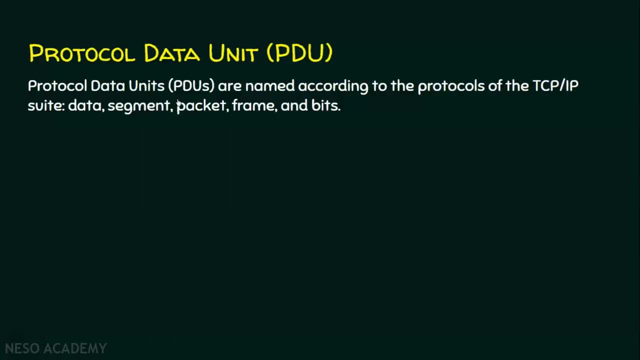 application layer. This is the TCP IP protocol suite. Now we will see what is PDU. that is, protocol data unit. Protocol data units are named according to the protocols of the application layer or the TCP IP suite. It means the PDUs can be data. 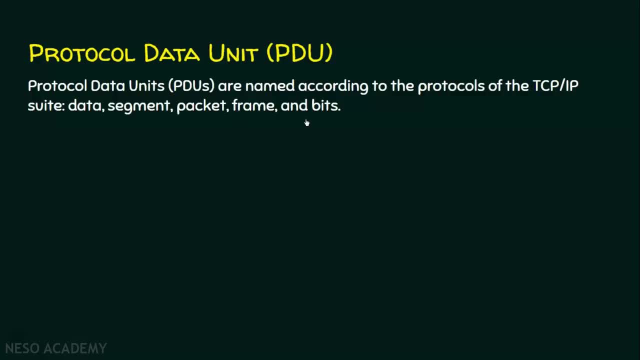 segment, packet, frames and bits. If you don't understand anything, just see this. Whatever the user generates, that is, from the application layer, that application layer information or that application layer PDU is called as simply data. So application layer PDU are simply called as data With application. 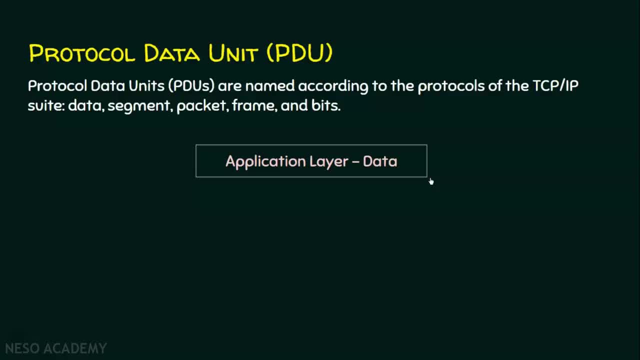 layer data, we will be obviously adding the transport layer header information. So once the transport layer information is added with the application layer data, we will call that as segment. So the transport layer PDU is called as a segment. After adding the transport layer information, we will be adding the network layer. 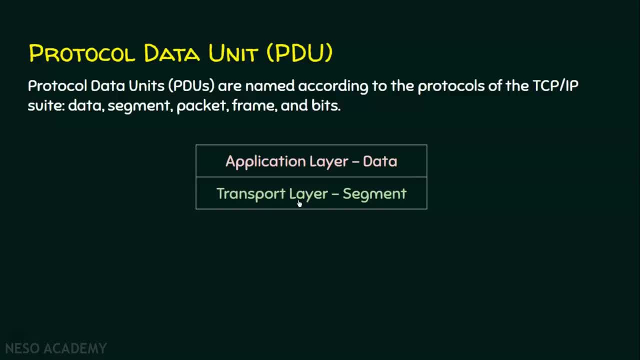 information. Once the network layer header is added we will call that as packet. So the network layer PDU is called as a packet. Now with this network layer we will be adding the data link layer part, that is, the header and the. 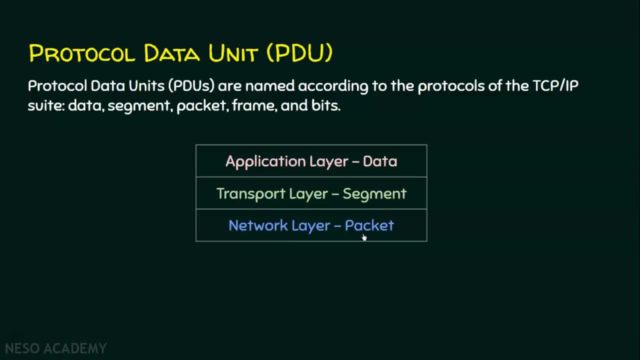 trailer. So with the packet we will be adding the header and the trailer in the data link layer. After adding the header and the trailer to the packet, the data link layer PDU is called as a frame. Now these frames are converted into zeros. 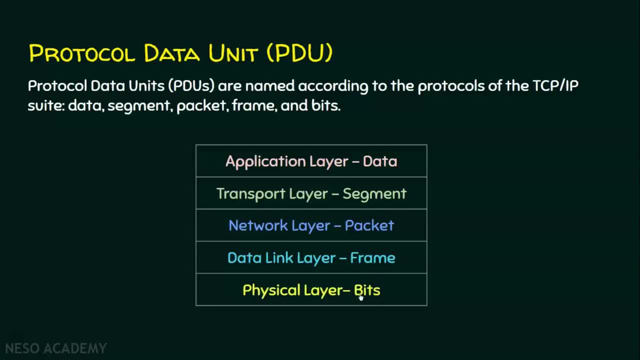 and ones in the physical layer. So the physical layer PDU, are called as bits. The application layer PDU is called as data. the transport layer PDU is called as segment. the network layer PDU is called as packet. the data link layer, PDU, is: 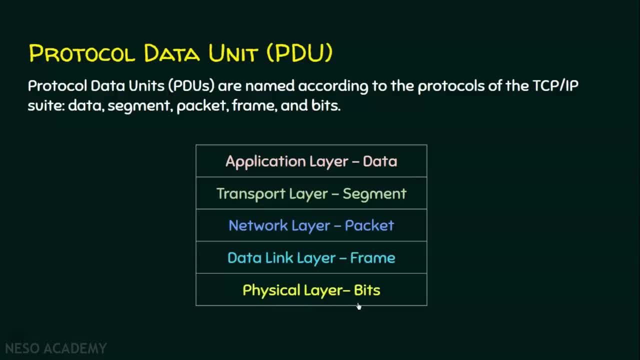 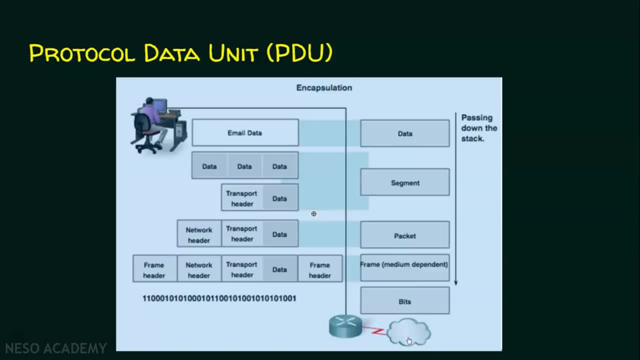 called as frame and the physical layer, PDU, is called as bits. We will see an example now. So in this example there's a user who's accessing a mail server somewhere in the internet. So there is a mail server. let's assume this is. 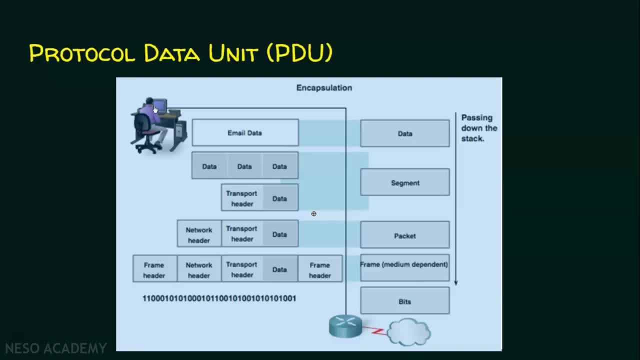 gmailcom. He has opened gmailcom in his browser and he is generating the application layer data. So this email data, whatever he is generating, is simply called as data in the application layer. So we can say, the application layer PDU is called as data. 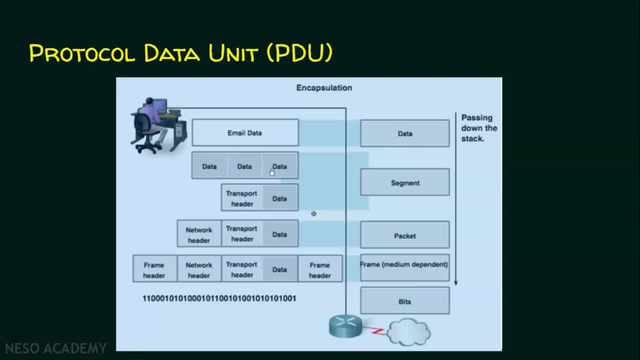 If it is a big data, obviously it is broken into smaller pieces. Now each of these smaller pieces are added with the transport header in the transport layer. Transport layer PDU is now called as a segment. Now this segment, this is actually the.